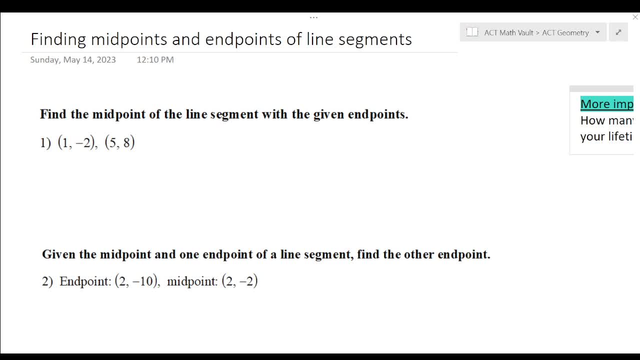 rethinking it. So if you're not thinking of it in terms of a formula, you're just rethinking it, reasoning yourself through it, maybe just with common sets, to remember the actual formula. it's: M equals, midpoint equals, and the final answer is going to be a. 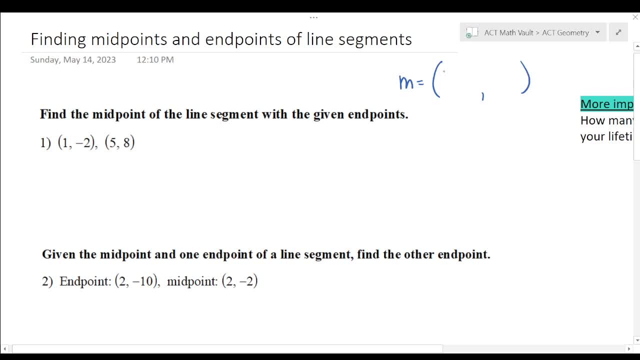 point. so it's just taking the average. let's say our two points are X 1, Y 1, X 2, Y 2. if our two points are X 1, Y 1, X 2, Y 2, then we'll have X 1 plus X 2 over. 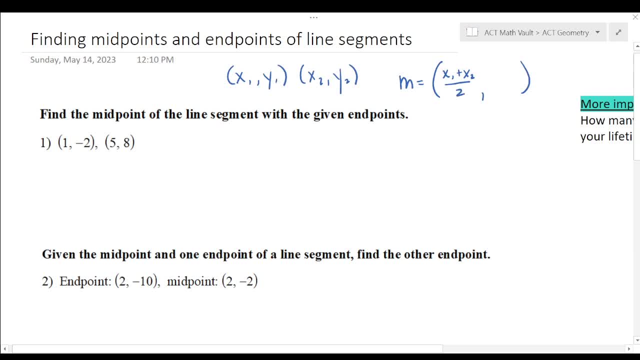 2, aka averaging the two X's and also taking the average of the two Y's. that will give us our final answer. so you really don't have to memorize the formula. formula for this, as long as you're thinking about it in terms of just taking the average of the 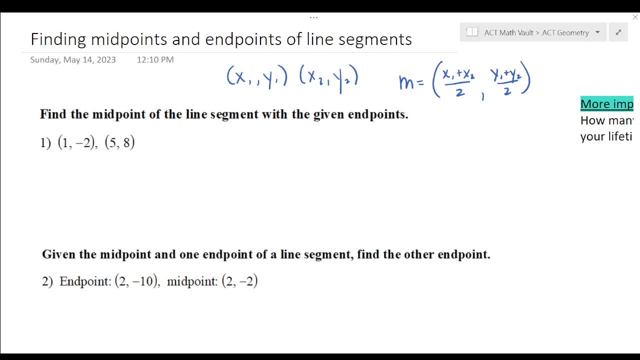 X's and the average of the Y's. if you look at a visual say of these two points makes a little bit more sense. why taking the average just makes sense. so one negative two is one of our points, and then five, two, three, four, five, two, three. 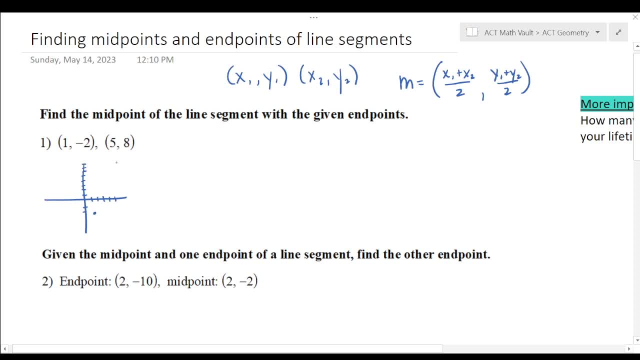 four, five, six, seven, eight. here's the other one. okay, so that line segment, you know, looks like this. we have to figure out where approximately is that that dot? well, it kind of looks like it's a or three. problem is: is you really need to know the exact point in some? 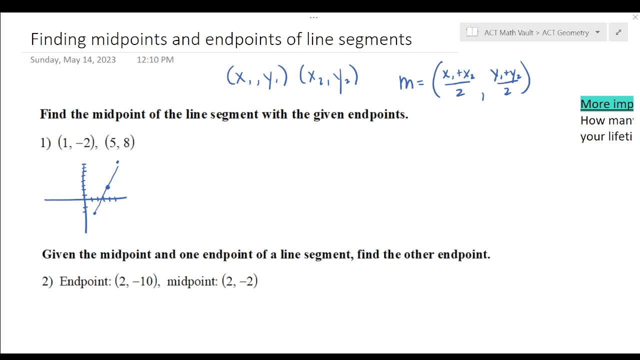 situation. so in this case, taking the average member of the X's, that would be like a shaped number, and then again we're going to do that again by taking the average up to about 6x. now again, this is not the ideal, that right, and I'm going to. 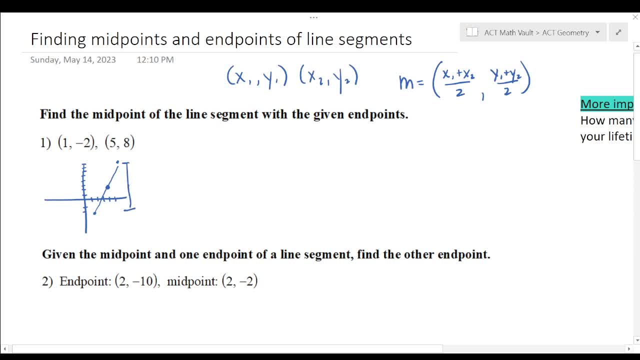 make sure this is my way of doing this. if you could view this graph on your own the other way around. so let's take this right. so the average of the two Y's is thinking: how am I going to set this up where I go? one plus five over two is the first part. 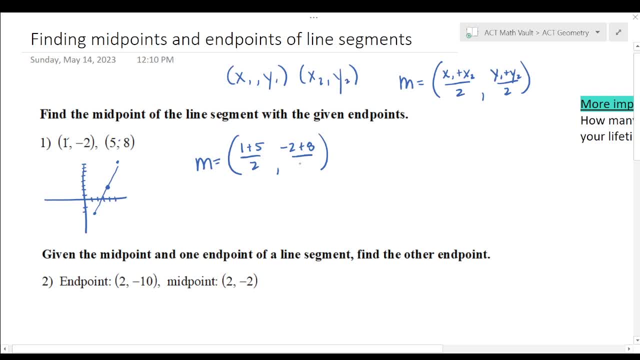 and negative. two plus eight over two is the second. m equals six over two, and then that is six over two as well. final answer is three, three. now some of you could probably do that in your head if you're under the gun for for time. for these you do not need to draw. 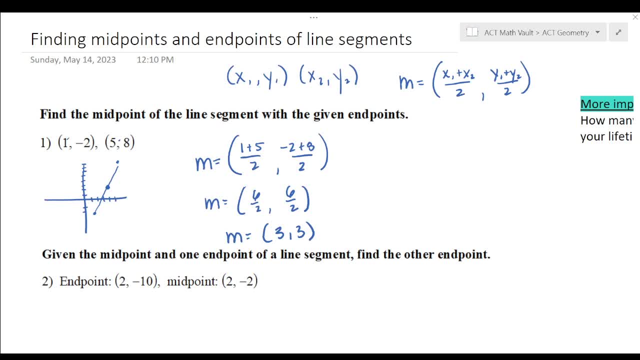 a picture and some of us don't even need to write out the formula. you're just thinking: what's the halfway point between one and five? what's the halfway point between negative two and eight, which is a little trickier, but knowing that you could just add them and divide by two makes it a 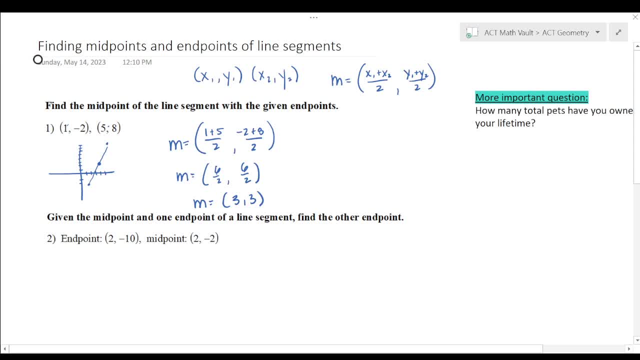 lot faster, but the ACT is known to make this a little more complicated when they're saying: okay, we'll tell you this end point and we'll tell you a midpoint, but now you have to decide what the final end point is. so how do you go backwards? okay, if we are given an end point. 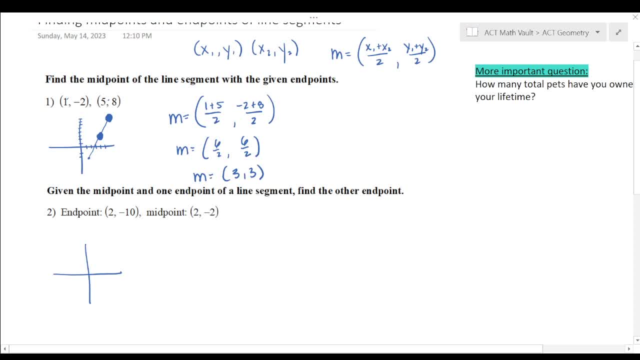 I'll draw out the, the visual, just in case this might be what sticks with you. uh, we go two and then let's say this is negative 10, down negative 10 or down 10. they're saying the midpoint is that two one, two negative two. okay, so two, two, two, negative 10. well, some people might be able to. 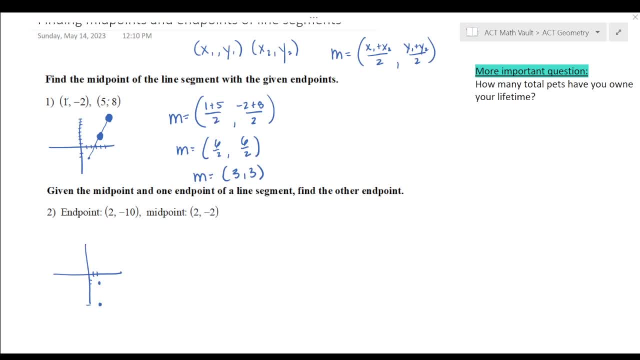 just start counting units and observing that, hey, if these are both on two, then maybe we could just start counting units, you know, from one to the next, but let's do it a little bit more scientifically. um, so, if we know that m is equal to remember x one plus x, two over two, y one plus y, two over two. 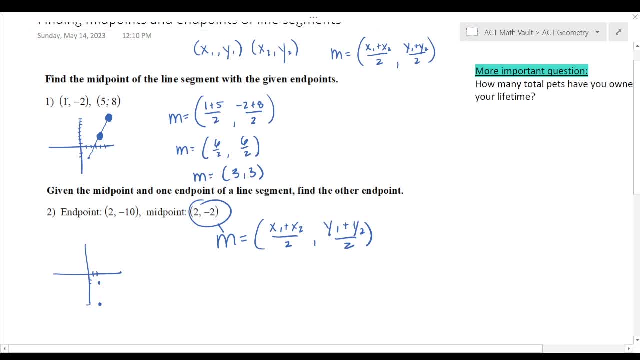 can't I set this equal to m and call this two and negative. two is equal to. now we have one point: x one, y one, let's call it. we have one of those and that is two and that is negative 10, and then just call the other parts, the other, you know, x two and y two, the unknowns. so really, I'm solving. 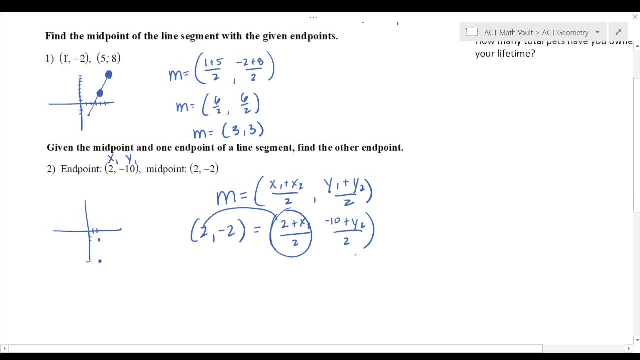 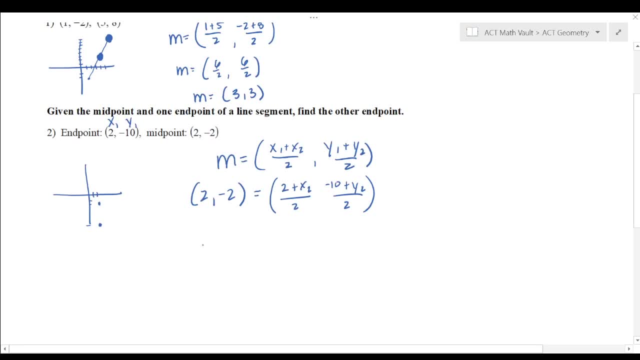 for you know, setting this equal to two, setting this equal to negative two. so I can do that as a separate step down here. just two plus x over two equals two, and then negative two equals negative. 10 plus y, two over two. this will help me solve for the unknown, so I can just call the other parts. 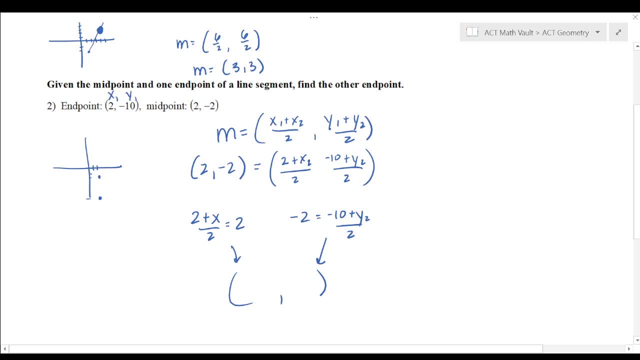 of my x- y pair of the other endpoint. so the way I can solve for that is if I multiply by two on both sides, those twos will cancel. I'll get two plus x equals four. so x is equal to two. okay, and uh, right here I can do the same times. two times two. we get negative four equals negative 10 plus y. I'm adding: 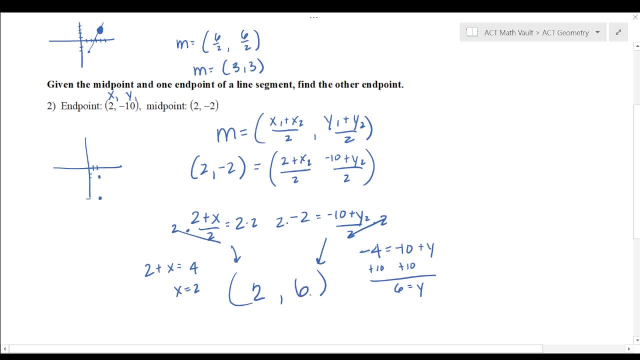 10. I'm adding 10, that's six equals the y. so now I know the other endpoint and hey, that actually makes sense, because if this is eight units down from one to the next, isn't the other endpoint going to be eight units up up there, two, six does make sense, okay. 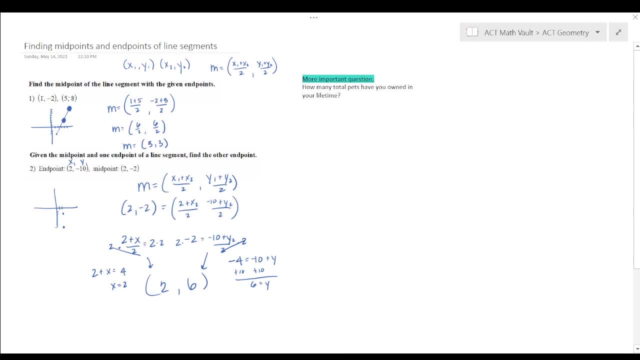 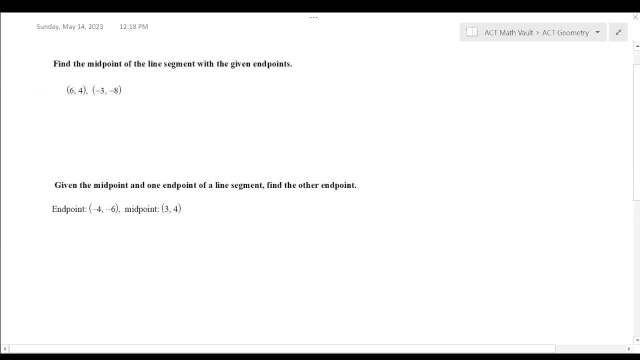 um. so let's think about some practice problems for you. try these one of each kind again, and I will reveal the answers in about one second. feel free to pause the video. here they are, so you actually end up getting a well mixed number. or you could call that three halves for the x in the first one, um, and then